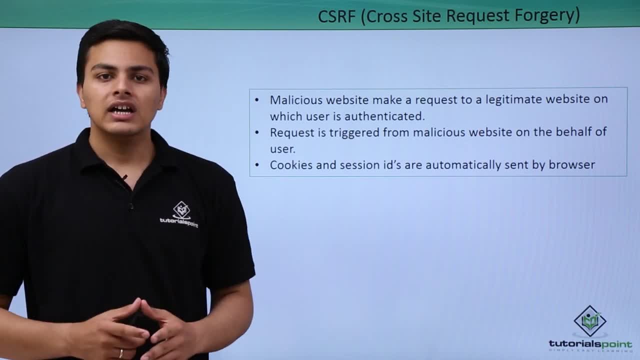 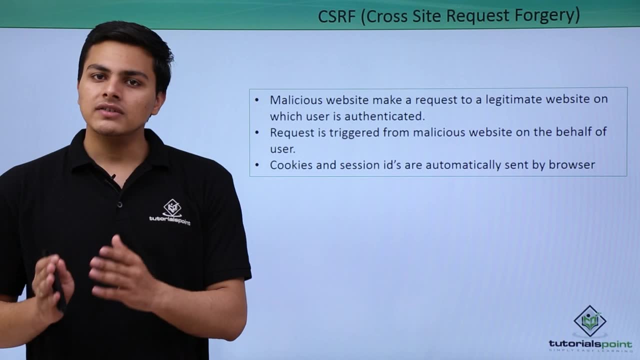 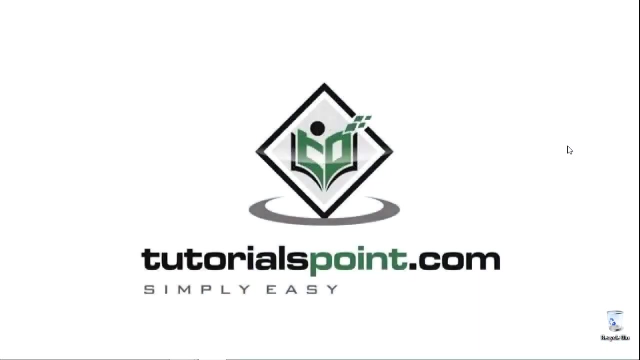 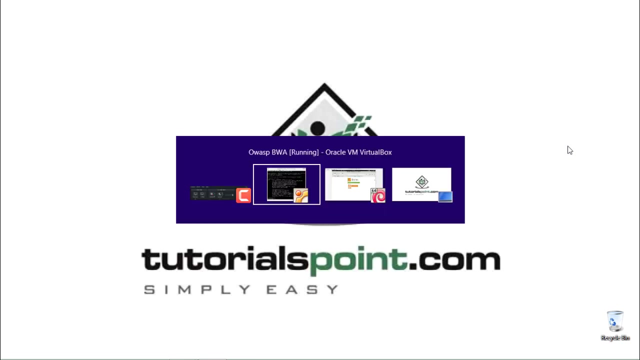 So the session IDs, cookies, tokens are all sent by users Browser to that legitimate website if the malicious website make a request. Now let's see how CSRF attack works. Now let's have a look at basic CSERF attack. The first thing we have to do is we have to start our OWASP broken web application, which we usually do all the times, and here you will see that my OWASP broken web application is up and running. 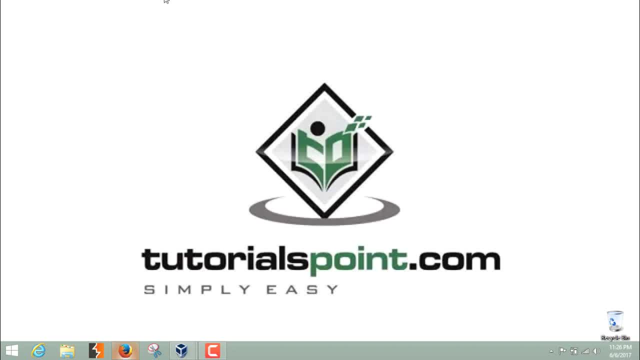 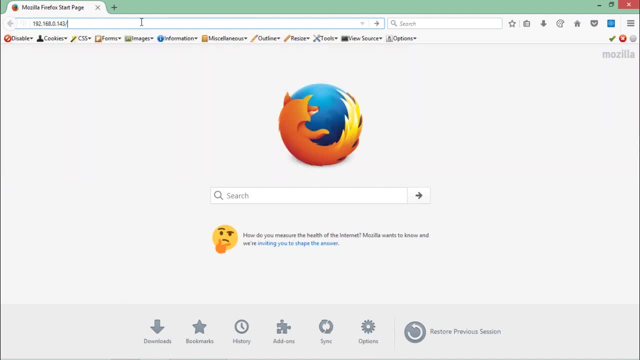 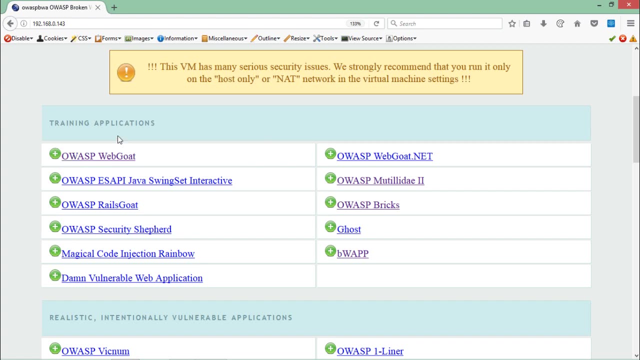 So let me open the OWASP broken web application Now. this time we have to use this web application, OWASP WebGoat. So if I just click over here, it asks us for the username and the password. So the username is guest and the password is guest. 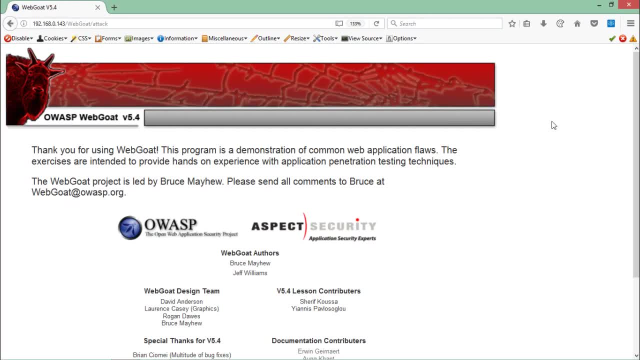 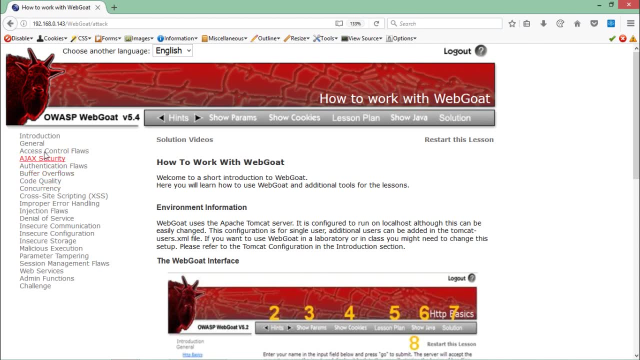 Click on OK. So here you will see the OWASP WebGoat web application. over here, start web goat and on the left hand side you will see lot of challenges. let's go here, cross head scripting, and here you will find one challenge called as cross site. 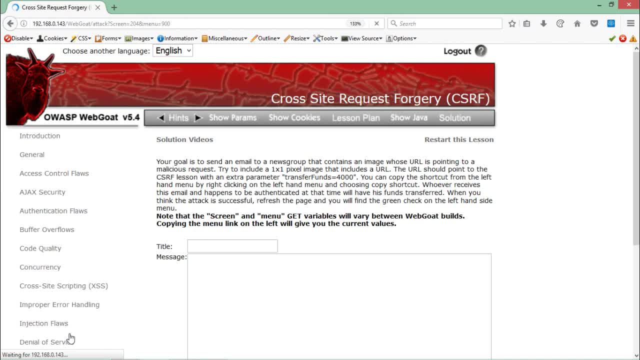 request forgery or csurf. let me open this challenge. so what we have to do is we just have to assume that we are a normal user, we are a authenticated user and we are logged in. so now what we have to do is we actually have to create html page, or we actually have. 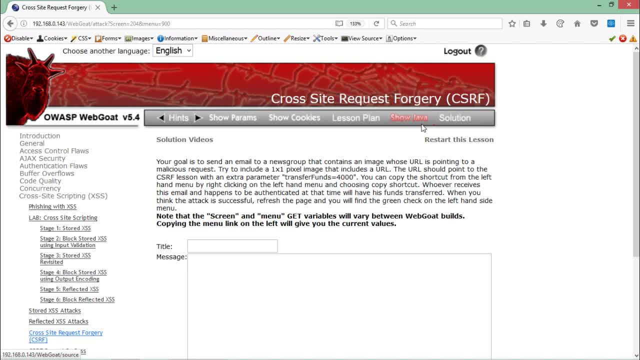 to create html page and inside it we have to create an image tag which will be hidden, so that image tag will actually points to this url. and in that image tag we have to pass additional parameter called as transfer funds. so if any user like me, i am authenticated user here as web goat. so if an attacker will 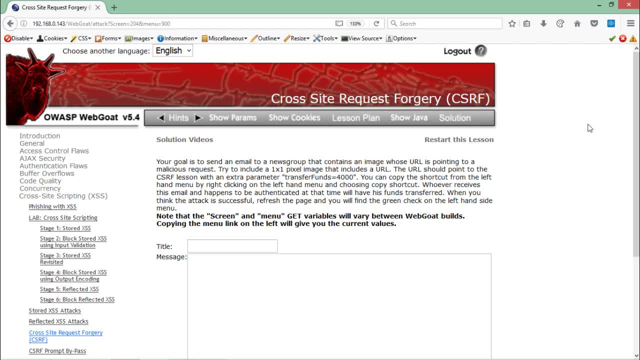 send me the link of its web page. so if i just open its web page, then a transfer of 4000 rupees will be done from my web goat account. so this is the challenge. so here you can see. your goal is to send an email to a news group that contain as html page and html page, and 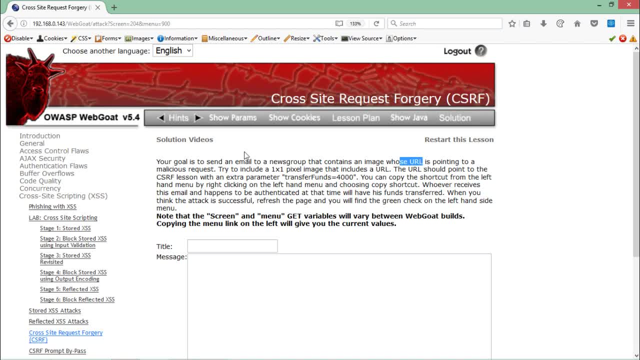 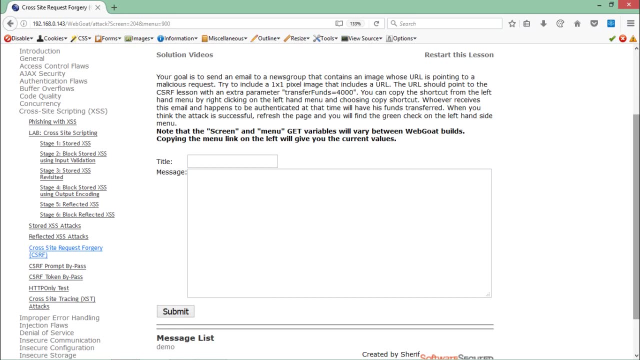 html page that contain an image whose url is pointing to malicious request, so try to include 1 x 1 pixel image. the url should point to csurf lesson with an extra parameter called as transfer funds, and here you will see that they have given us something to store the 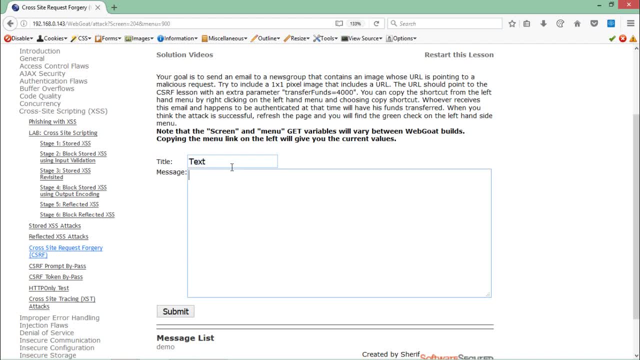 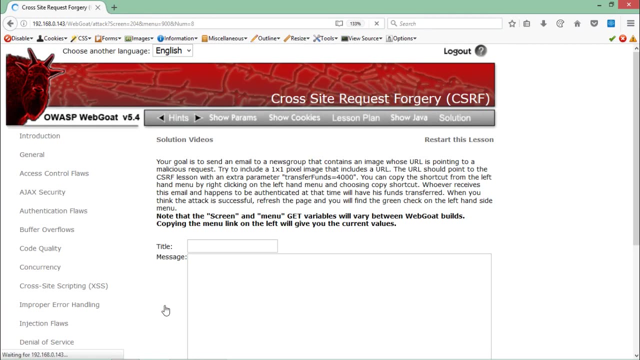 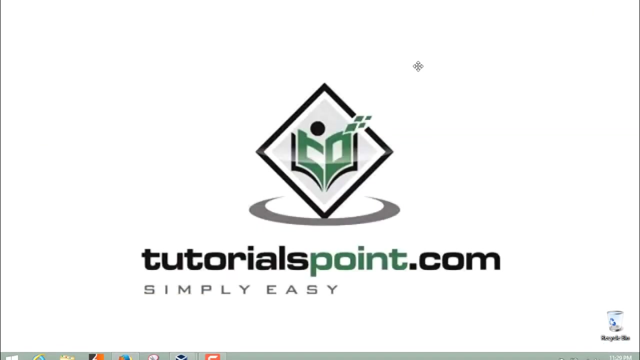 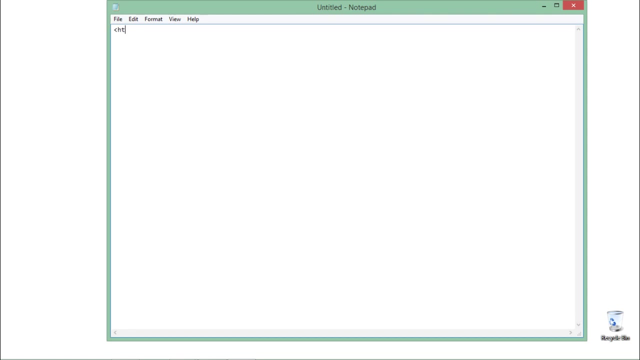 value, like if i just write here text: Hello, this is sample text, and now if I just click on submit, you will see that this text has been submitted and we can just read it content. Now let's create HTML file which will point to that CSRF URL. so height should be 1 and width should be 1, and the source: 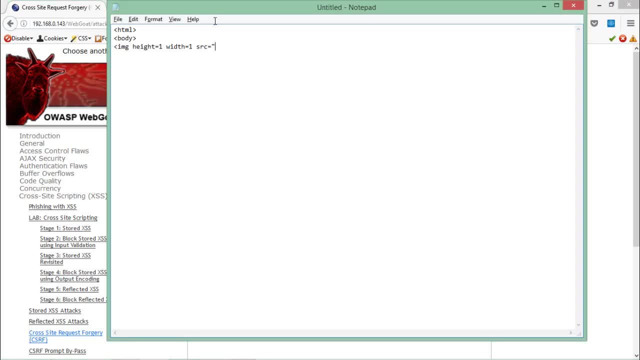 let me just copy this, Let me paste it over here. and what they want is they want an additional parameter called as transfer funds equals 4,000.. So here you will see that our HTML webpage is ready. Now one thing more so: there are different, different tags in the HTML which we can use to trigger the CSRF attack. 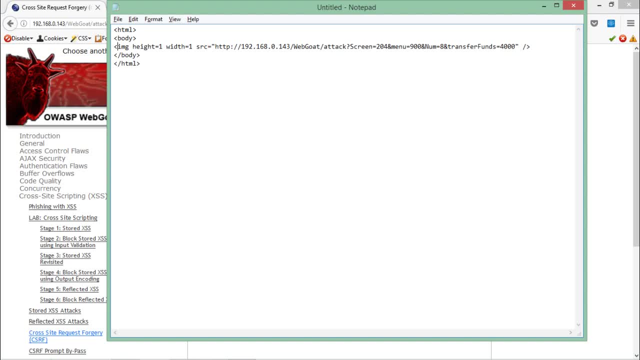 So the one is image, because the image tag contain a source and we can point the source to our CSRF web application. So we can also use iframe tag, because iframe tag also consist of this attribute source. Then we can also use script tag and few more.